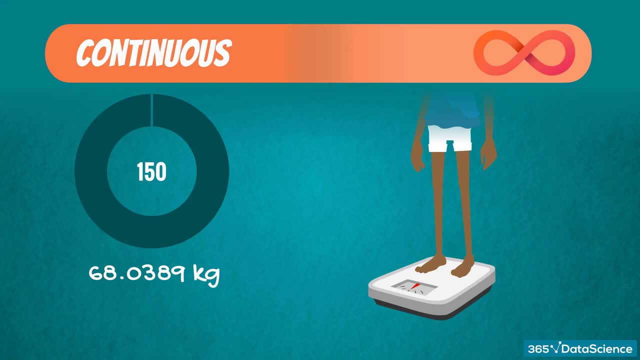 But this is just an approximation. If you gain 0.01 pound, the figure on the scale is unlikely to change, but your new weight will be 150.01 pounds or 68.0434 kilograms. Now think about sweating. Every drop of sweat reduces your weight by the weight of that drop. 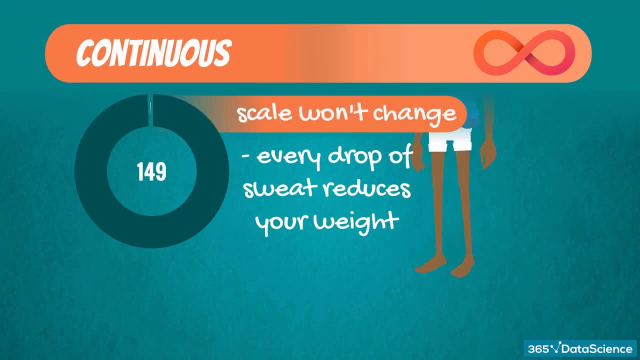 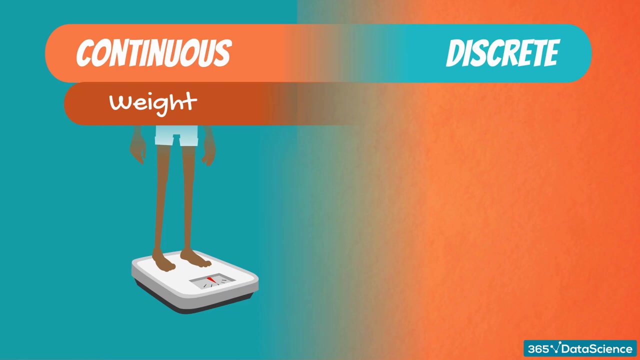 but, once again, a scale is unlikely to capture that change. Your exact weight is a continuous variable. It can take on an infinite amount of values, no matter how many digits there are after the dot. To sum up, your weight can vary by incomprehensibly small amounts and is continuous. 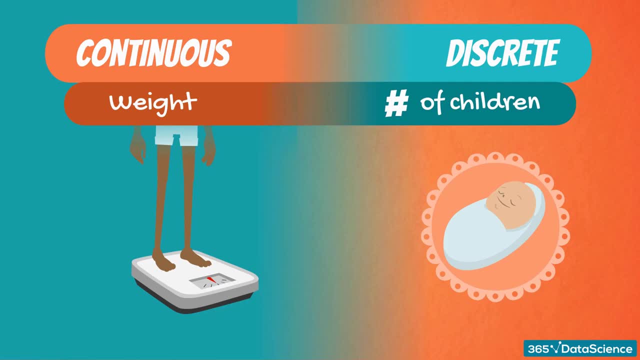 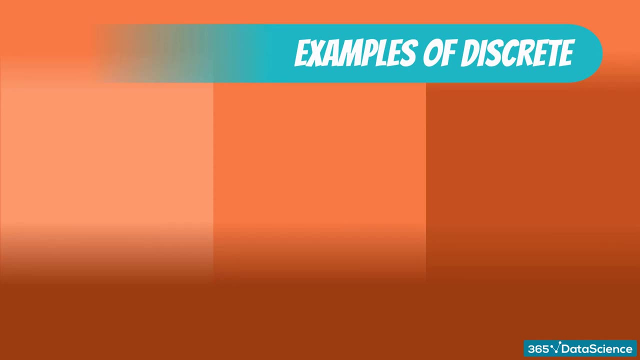 while the number of children you want to have is directly understandable and is discrete. Just to make sure, here are some other examples of discrete and continuous data. Grades at university are discrete: A, B, C, D, E, F or 0 to 100%. 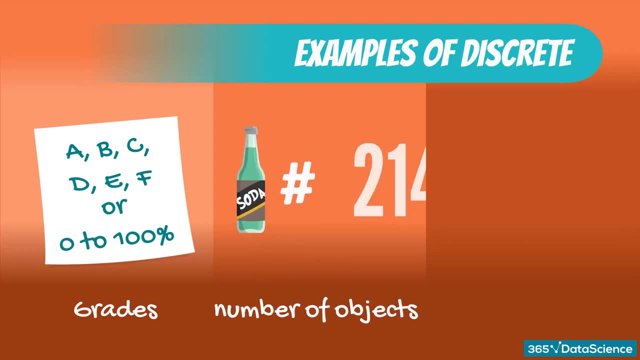 The number of objects in general, No matter if bottles, glasses, tables or cars, they can only take integer values. Money can be considered both, but physical money like bank notes and coins are definitely discrete. You can't pay $1.243.. You can only pay $1.24.. That's. 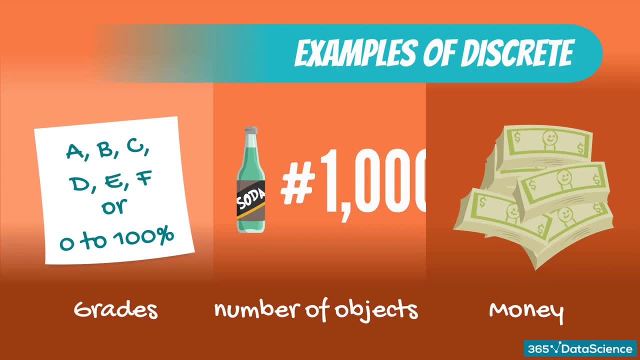 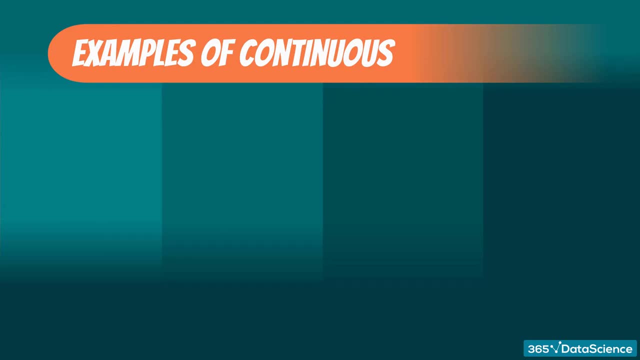 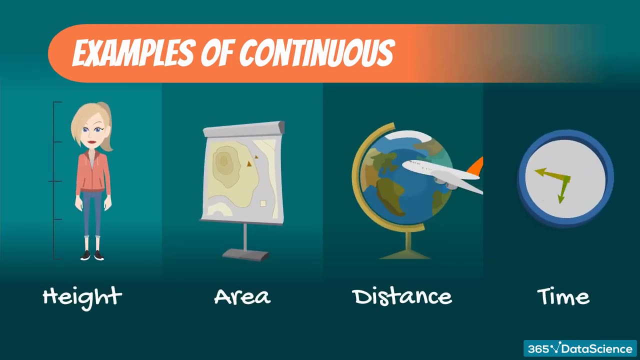 because the difference between two sums of money can be one cent at most. What else is continuous? Apart from weight, other measurements are also continuous. Examples are height, area, distance and time. All of these can vary by infinitely smaller amounts. 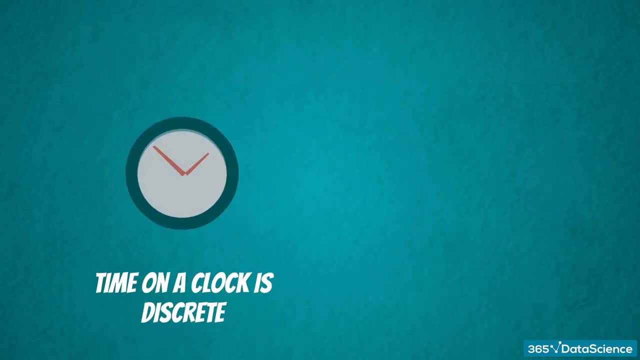 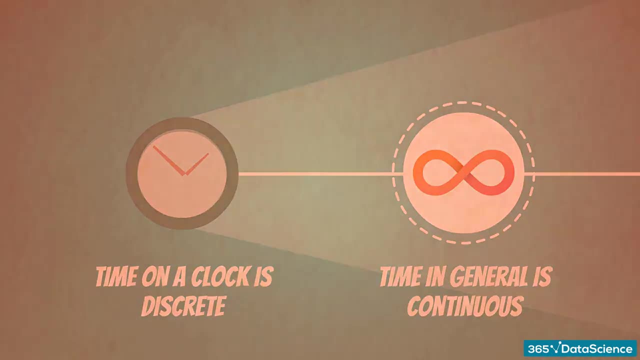 incomprehensible for a human. Time on a clock is discrete, but time in general isn't. It can be anything like 72.12345.. We are constrained in measuring weight, height, area, distance and time by our technology. 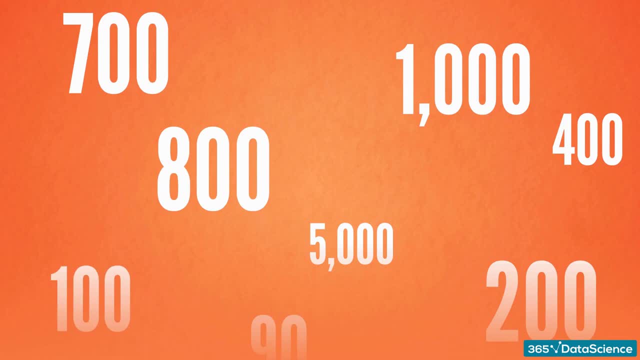 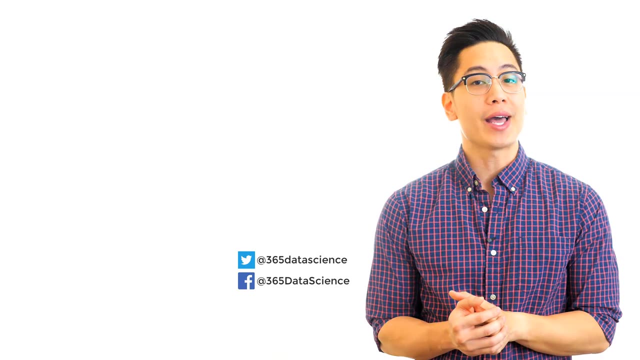 but in general, they can take on any value. Alright, these were the types of data. If you found this video interesting and want to gain an edge in your career, make sure to like, comment and subscribe, And don't forget to check out some of our other videos for another quick win in the data science skills department.